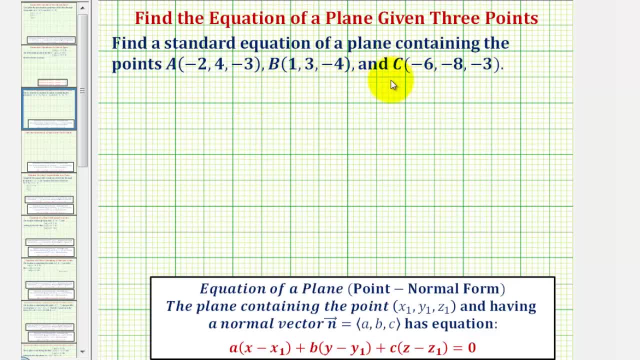 the plane, Then, if we find the cross product of those two vectors, it would give us a normal vector to the plane. Before we do this, though, let's take a look at this in space. Here we see the yellow plane that we're trying to find the equation of, and these three points. 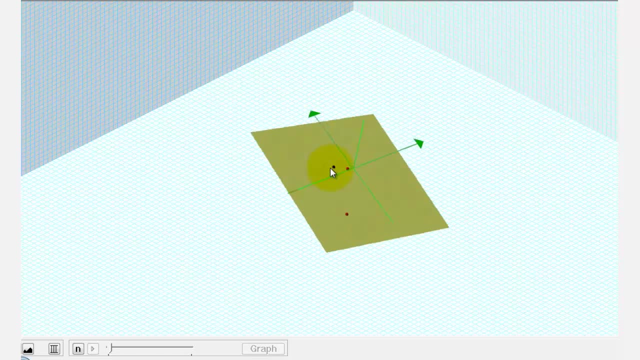 are the points given that are in the plane. Point A is in blue and points B and C are in red. So, again, our first step will be to find vector A- B and vector A- C, which will give us two vectors in the plane. 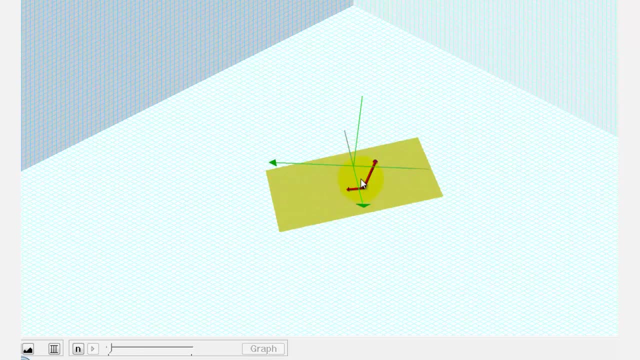 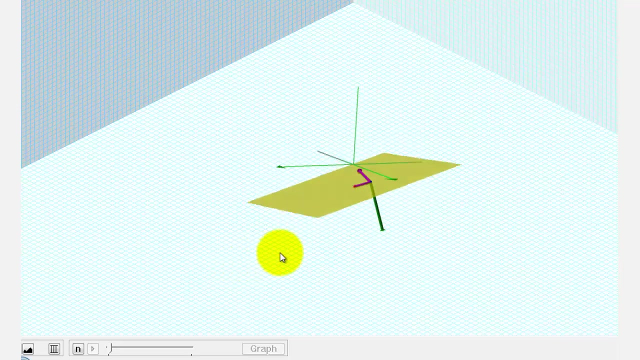 Those two vectors would look like this: Once we find these two vectors, we'll find the cross product of these two vectors, which will give us a normal vector. So when we cross these two vectors, the normal vector would look like this: So once we find this normal vector by determining the cross product, we have all the information. 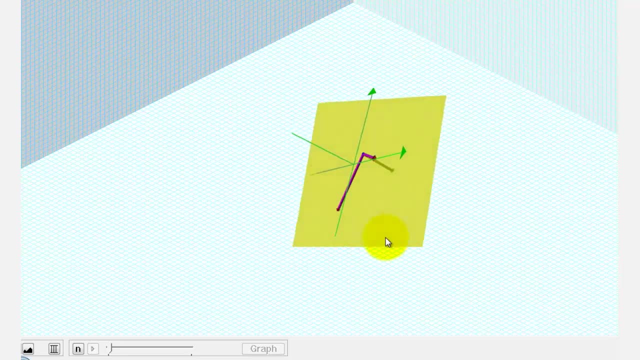 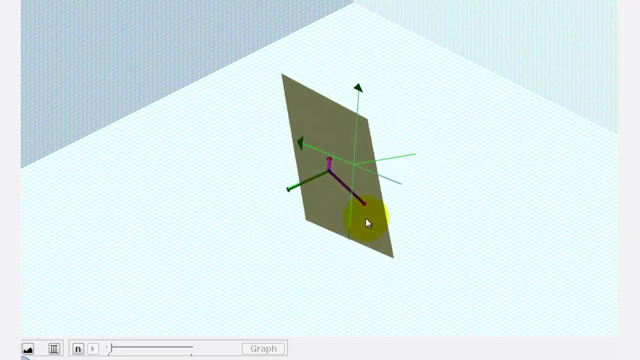 we need in order to find the equation of this plane. We'll use the component form of the normal vector and we'll select one of the three points to determine the equation of the plane. So now let's go find the equation of this plane. 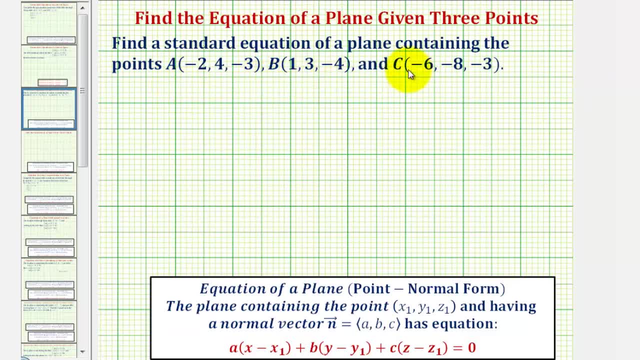 We'll begin by determining the equation of this plane. We'll use the component form of vector A B and vector A C in component form. To write these vectors in component form, we'll take the coordinates of the terminal point and subtract the coordinates of the initial point. 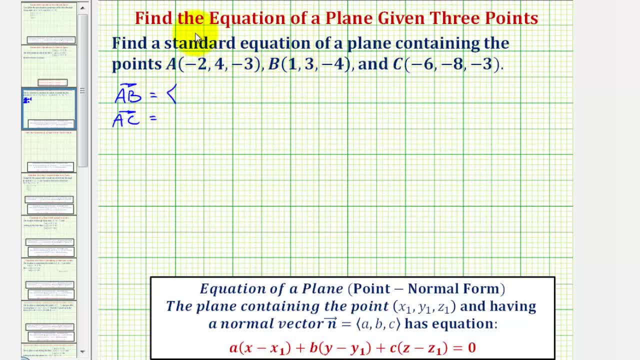 So vector A B in component form would have an x component of one minus negative two, that's positive three, a y component of three minus four, that's negative one, and a z component of negative four minus negative three, which is negative four plus three or negative one. 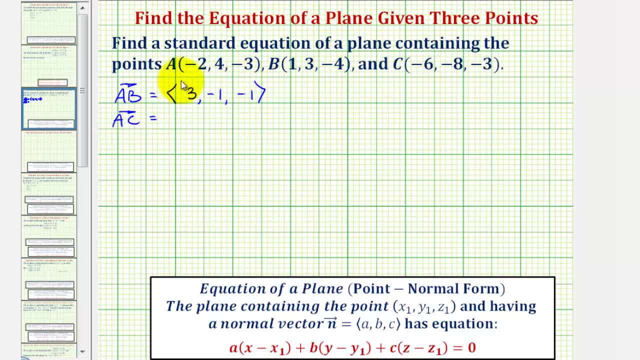 And now for vector A C. the x component would be negative six minus negative two, which is negative six plus two, or negative four. The y component would be negative eight minus four, that's negative twelve, And the z component would be negative three minus negative three, which is zero. 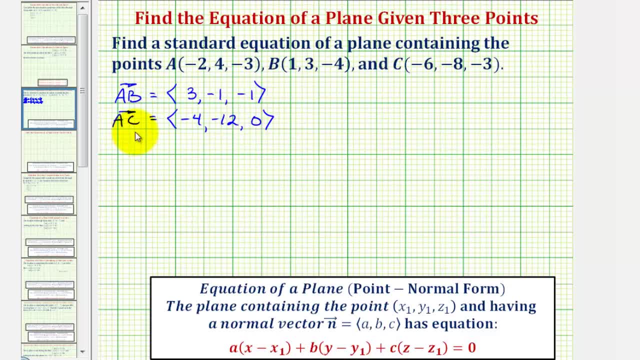 Now to find the normal vector. we could cross these two vectors, but we could also use any scalar multiple of vector A, B or negative four. So we'll use the common vector of vector A, B or negative four. So we'll use the common vector of vector A, B or vector A C. 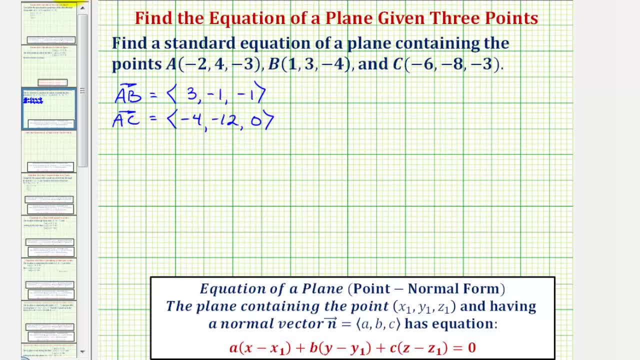 So let's use a simpler vector rather than vector A C. Notice how, if we used negative one fourth times vector A C, this vector would still be in the plane. it would be in the opposite direction and would have one fourth the magnitude. 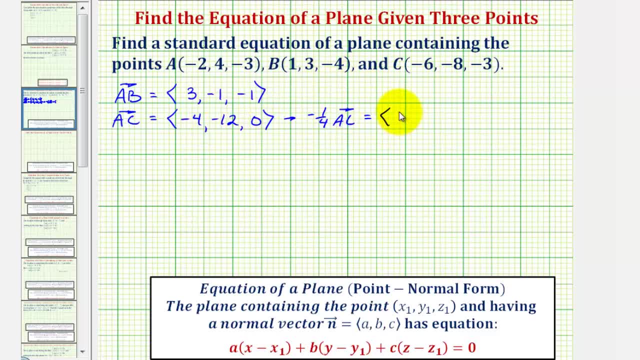 This would be equal to the vector with an x component of positive one, a y component of positive three and a z component of zero. This will make finding the cross product easy. But notice how, because we did change the direction of this vector because of the negative one, 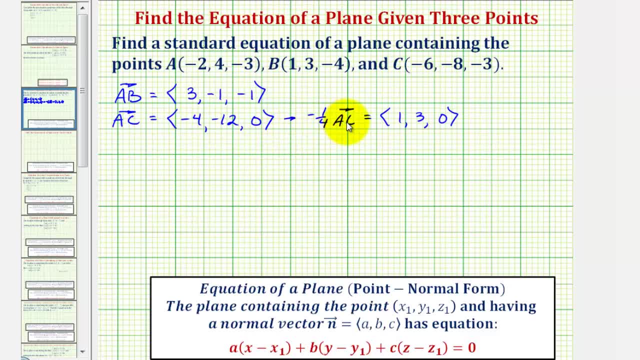 fourth, this would give us a different normal vector than the one we saw graphed in 3D. So now we'll find the cross product of vector A, B and vector negative, one, fourth times vector A- C, which again will give us our normal vector to the plane. 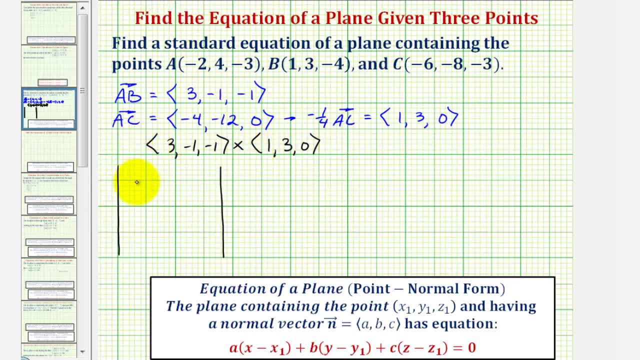 So we'll set this up as a three by three determinant, where the first row will be vector i, vector j and vector k. The second row will be the components of vector A- B. The third row will be the components from vector negative one, fourth times A- C. 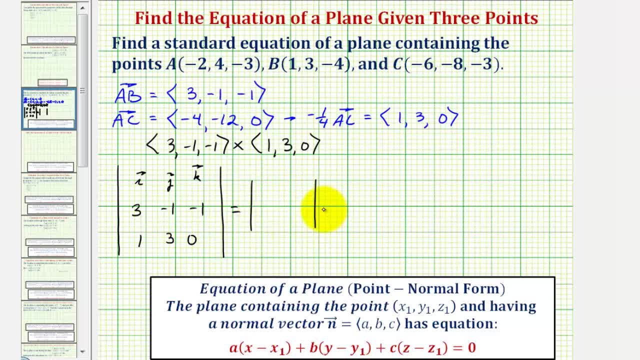 This will be equal to a two by two determinant times vector i, minus a two by two determinant times vector j, A two by two determinant times vector k. So to find the elements in this first two by two determinant, we eliminate the row and column of vector i. 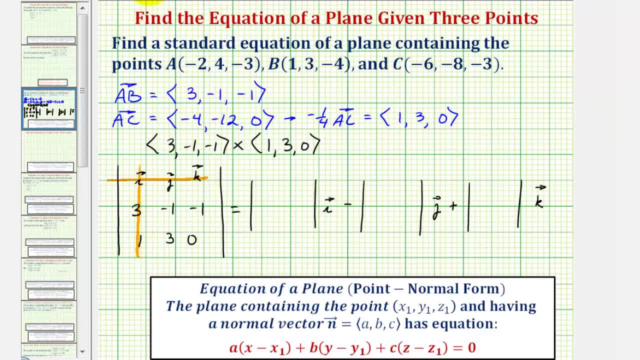 So we eliminate row one and column one. the remaining elements of the elements in this first two by two determinant To find the elements in this two by two determinant. we'll eliminate the row and column of vector j. So we'll eliminate row one and column j. 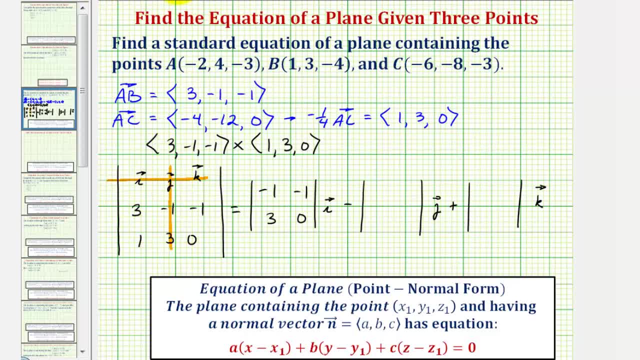 row one and now column two. The remaining elements are the elements for our two by two determinant And then, following for the elements here, we eliminate the row and column of vector k. So again, we eliminate row one, but also column three. 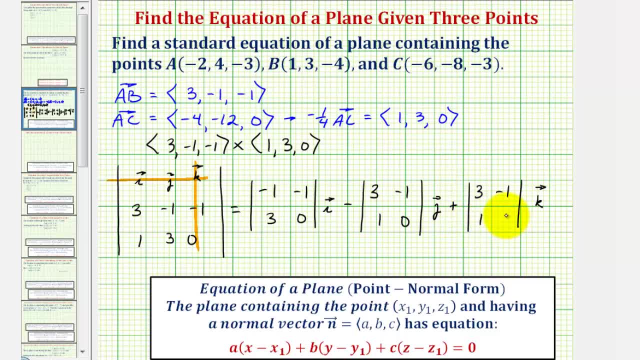 So the elements would be three: negative one, one, three. So now our normal vector, we'll call vector n- will be equal to: here. we have negative one times zero minus negative one times three. That would be positive three. so we have three i. 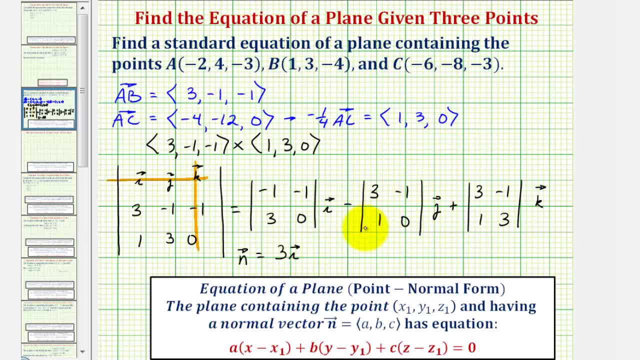 Here we have minus three times zero, minus negative, one times one. The value of the determinant is positive one, but we're subtracting, so it's minus one j or just minus j. And then here we have plus three times three. 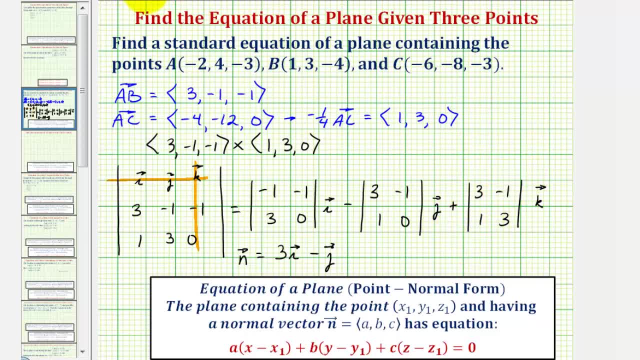 minus negative one times one. So that would be positive 10, so we have plus 10 times vector k. So in component form the normal vector would have an x component of three, a y component of negative one and a z component of 10.. 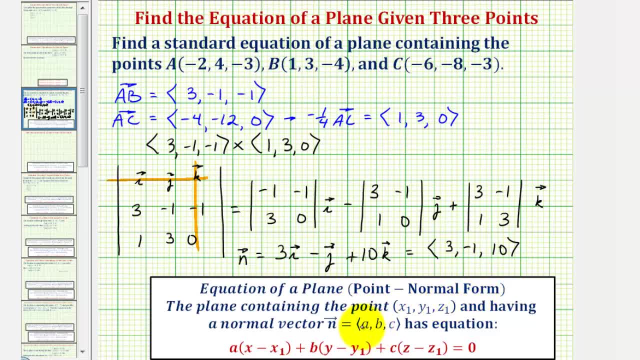 Now we have all the information we need to find the point normal form of our plane, which we'll then write in standard form. So we'll use the components of the normal vector and we can use any of the three given points. Let's use point b. 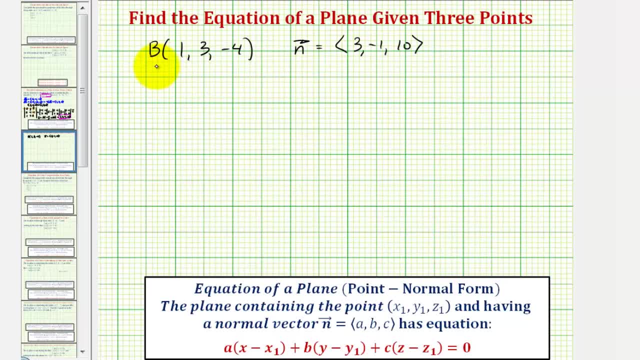 So let's find the equation of our plane on the next slide. So because point b is a point in the plane, we know that x sub one is equal to one, y sub one is equal to three and z sub one equals negative four. 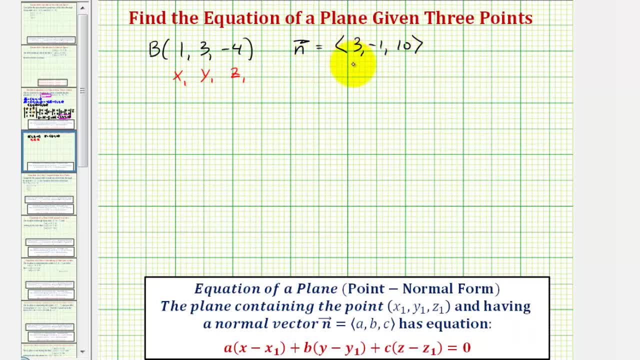 And because this is our normal vector to the plane, we know that a equals three, b equals negative one and c equals 10.. So the point normal form of the equation of our plane would be a, which is three times the quantity. 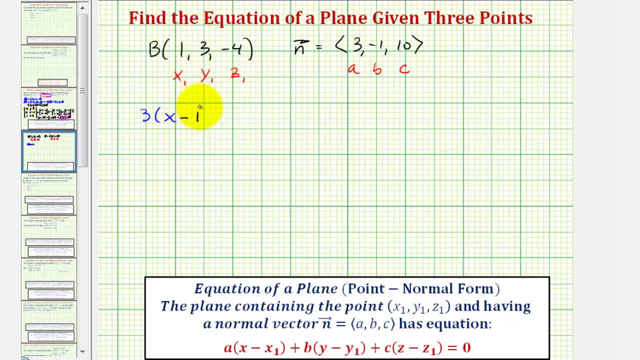 times the quantity x minus x sub one, so we have x minus one plus b. but since b is negative one, we have minus one times the quantity y minus y sub one, so we have y minus three, and then plus c or plus 10,. 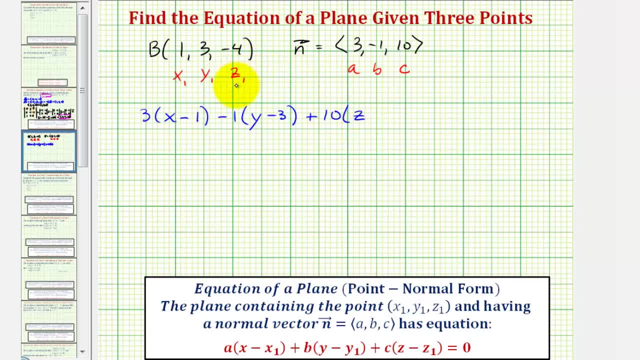 times the quantity z minus z sub one, which would be z minus negative four, which is the same as z plus four, equals zero. equals zero. Now that we have the equation in point normal form, we'll write this equation in standard form.